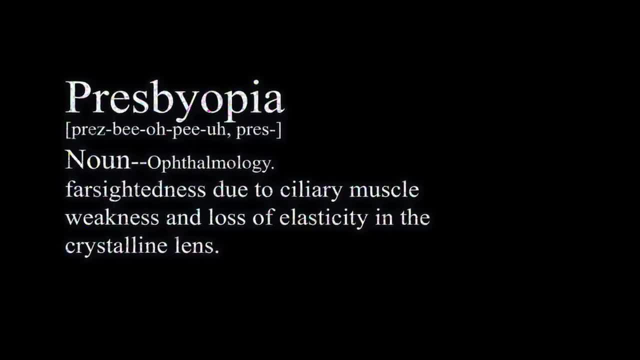 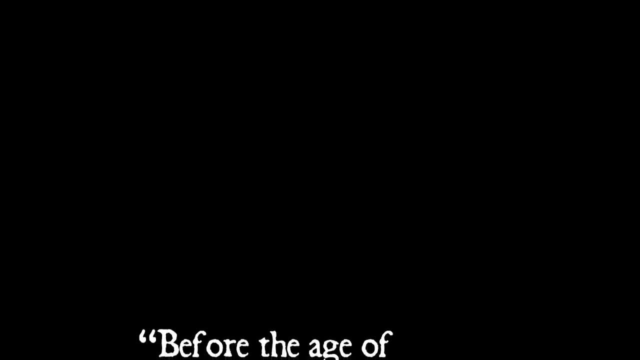 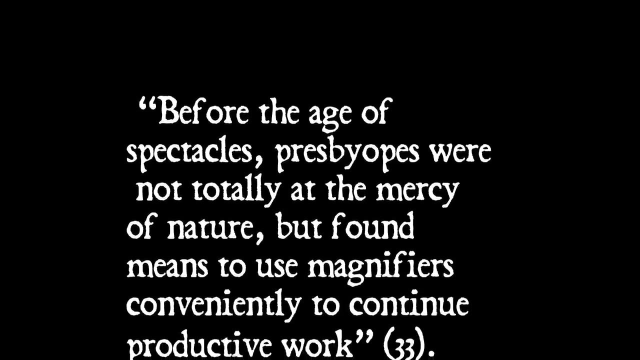 presbyopia, or farsightedness, an inevitable byproduct of aging that's plagued primates for millions of years. Historian Vincent Ilardi writes that before the age of spectacles, presbyopes were not totally at the mercy of nature, but found means to use magnifiers. 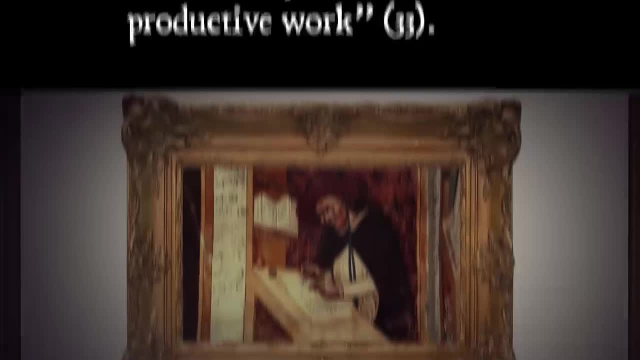 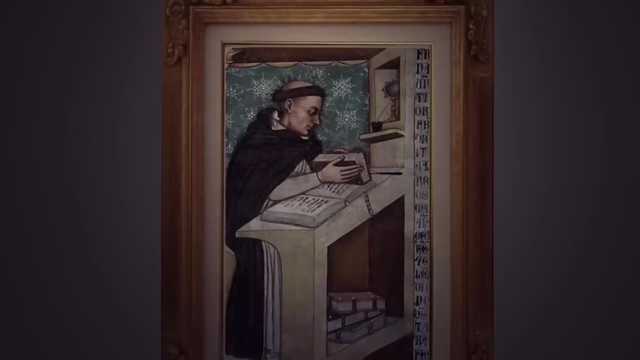 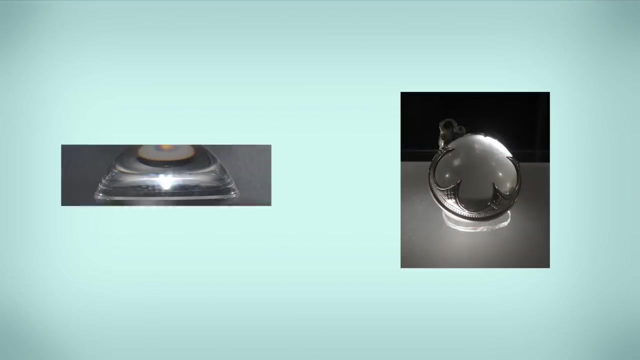 conveniently to continue productive work. Go back to the monastery in Treviso and you'll find a painting that shows one such magnifying lens. At that point, primitive magnifiers had been around for thousands of years. Excavations of Viking graves have uncovered the Visby lenses from the 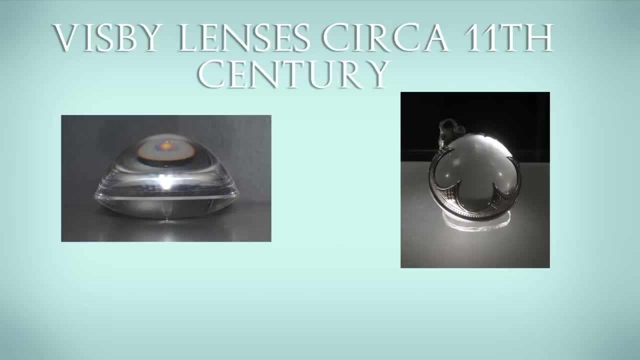 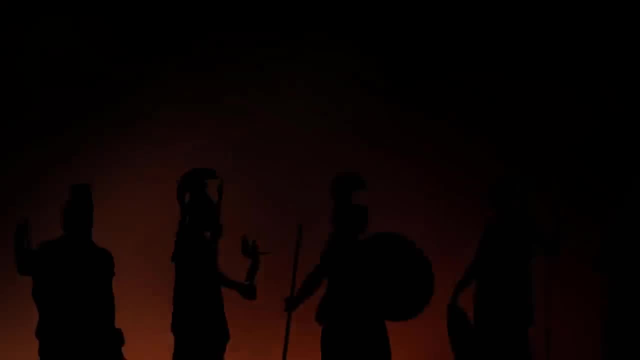 11th century. This is the first time presbyopes have been found to be used for magnifying purposes. They're perfectly ellipsoid crystals, probably used as reading stones or by craftsmen to see fine details. Other lenses are much older. The ancient Greeks and Romans had polished magnifying crystals. 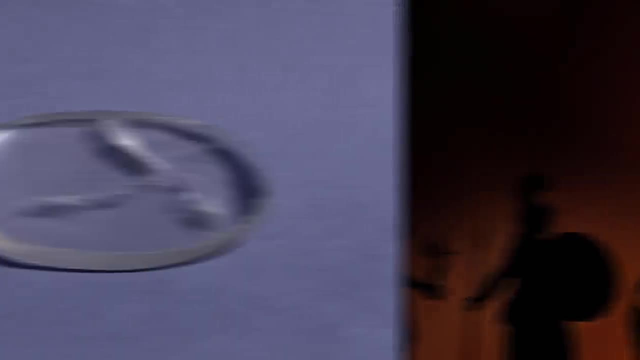 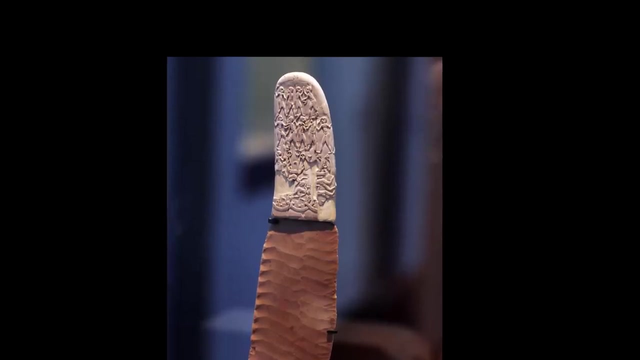 which they used to light fires, And the ancient Assyrian Nimrud lens dates back to 750 BC. Quartz lenses even existed 4,600 years ago in Egypt's old kingdom. Some scholars have wondered if Egyptian artisans used these lenses to make the magnifying lenses. In fact, the 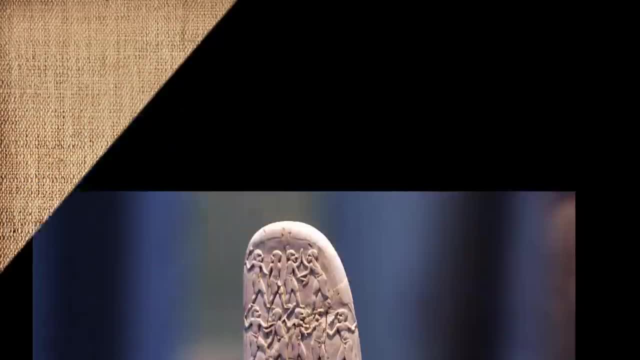 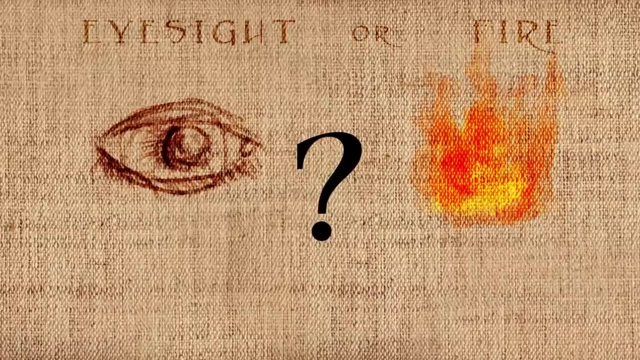 ancient Assyrians used these lenses to make the magnifying lenses, Although it's not clear that all of these ancient lenses were used to enhance vision. magnification was a well-established technology before glasses. In general, if you were farsighted, there was hope. 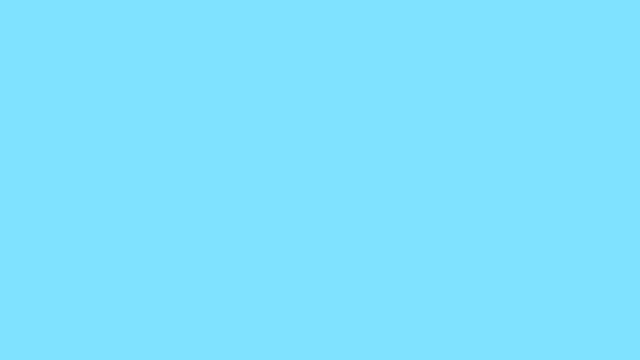 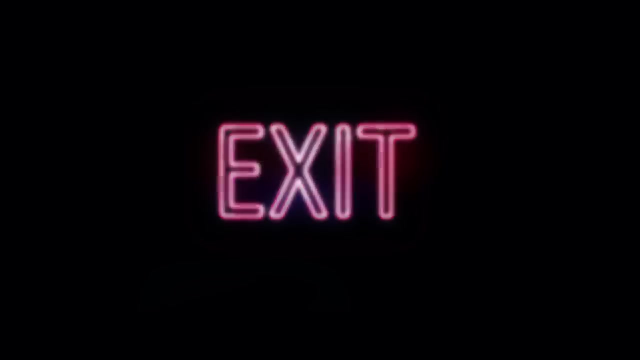 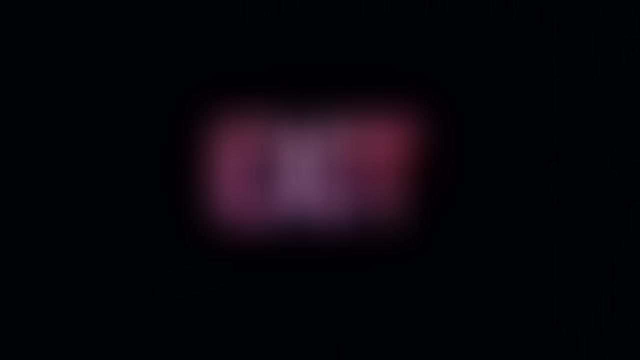 But what did nearsighted people do? Surely, if you're the kind of person that can't read an exit sign from 10 feet away, you'd have been useless in battle or seafaring. That assumption is probably correct. For instance, in the 1st century AD, the Romans excused an Egyptian weaver named Triphon. 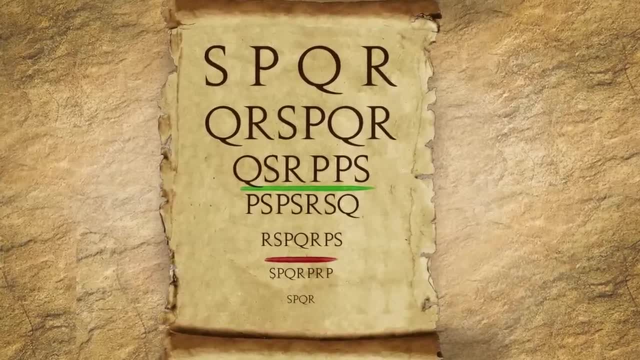 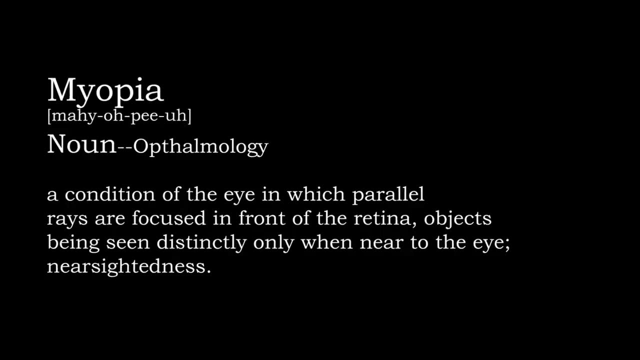 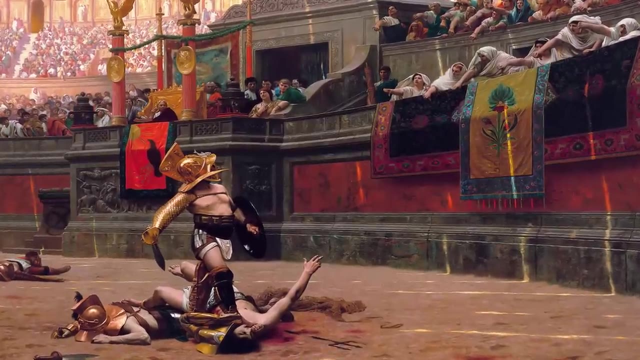 from military service for shortness of sight. If technologies existed to help people with nearsightedness or myopia, they were primitive and rare. Emperor Nero reportedly needed to watch gladiator games through a polished emerald that concentrated the powers of vision. Yet